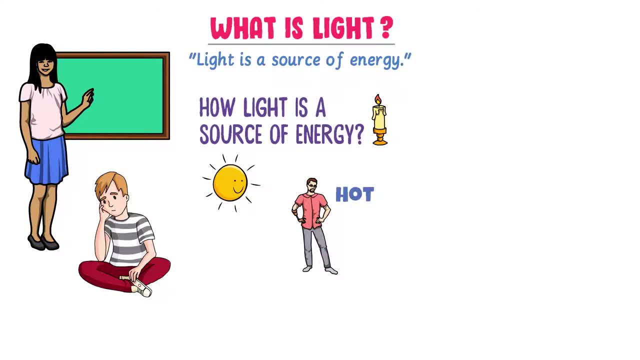 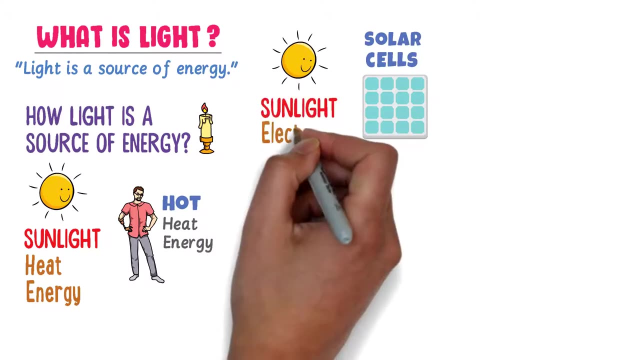 your body becomes hot. It means that your body absorbs heat energy from the sunlight. Thus we say that sunlight or light possesses heat energy. Secondly, we use solar cells or photovoltaic cells, which convert the energy of the sunlight to electrical energy. We can then 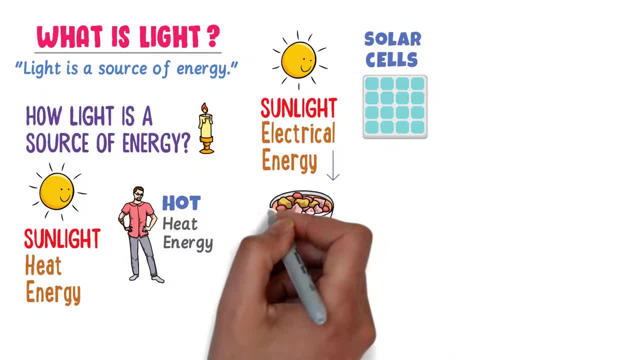 do different work using electricity, like heating food, heating water, etc. Thus sunlight or light is a source of energy, because it heats our food and water. Thirdly, the solar cars. In solar cars, solar panels are used to recharge battery and run a car. Thus sunlight or light is 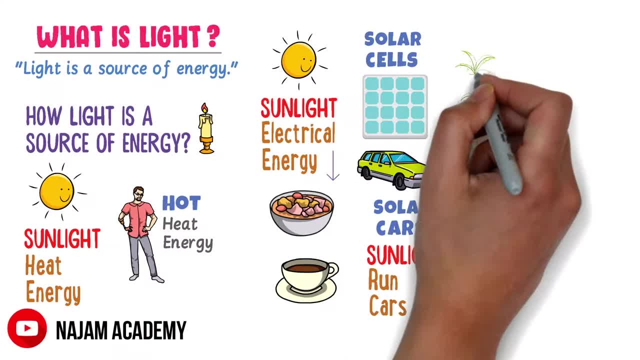 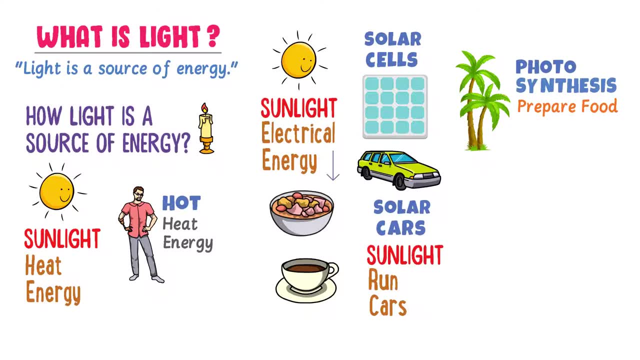 a form of energy that run our cars. Fourthly, photosynthesis and plants. We know that plants prepare their own food by the process of photosynthesis. For example, carbon dioxide plus water combined together in the presence of sunlight to form glucose- C6H12O6. 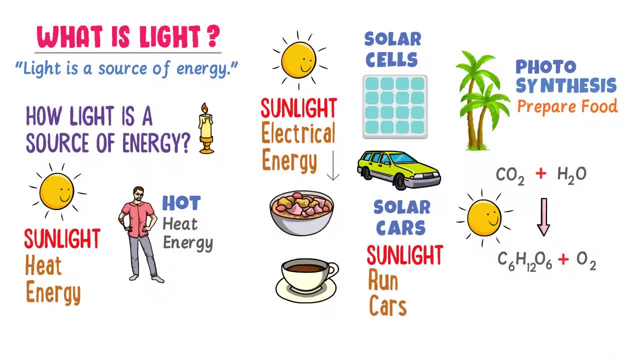 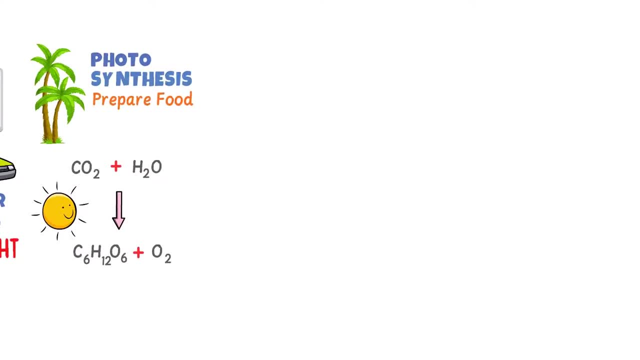 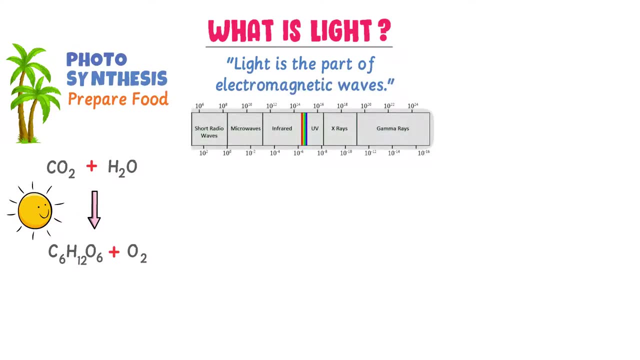 is the food or energy of the plant. Thus, sunlight or light is the source of energy. Therefore, remember that light is a source of energy. Now, the second most common definition is that light is the part of electromagnetic waves, just like hand is the part of our body. We know that. 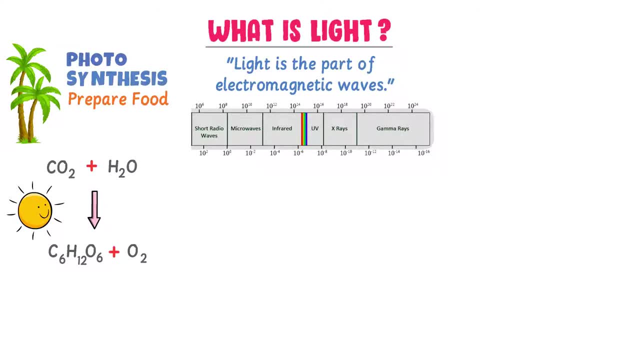 an electromagnetic spectrum. there are different waves, like radio waves, microwaves, x-rays and gamma rays. The visible light is the part of our body and the visible light is the part of our body, and the visible light is also present in this series of electromagnetic waves. Therefore, 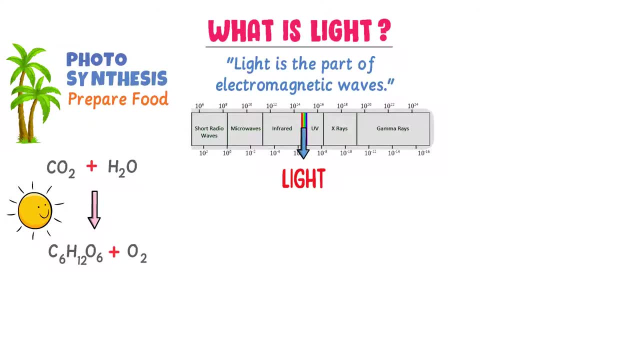 we say that light is the part of electromagnetic waves. Now, what are electromagnetic waves? Well, electromagnetic waves are the waves that produces due to the perpendicular oscillations of electric field and magnetic field. To learn more about electromagnetic waves, watch our lecture and its 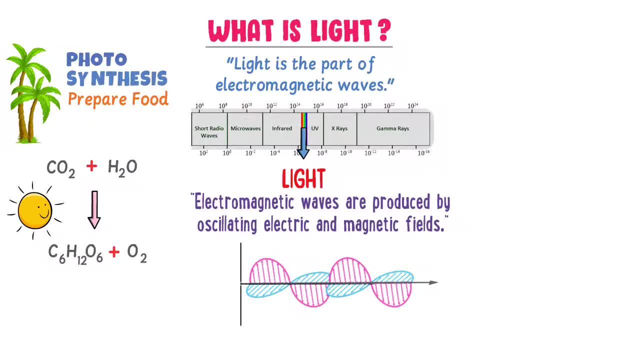 link is given in the description. Now consider that if electromagnetic waves are the part of our body, electric field oscillates in x-direction and magnetic field oscillates perpendicular to it in y-direction, then electromagnetic waves are produced in z-direction. So perpendicular oscillations of electric field.